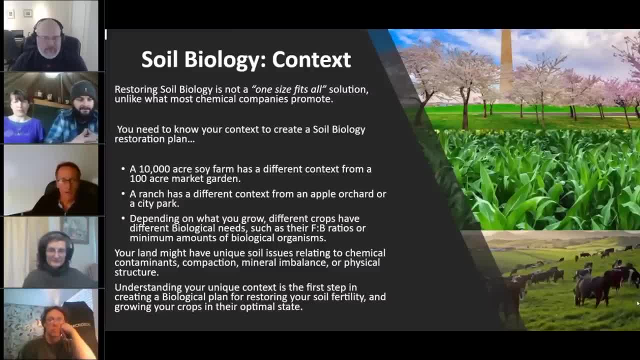 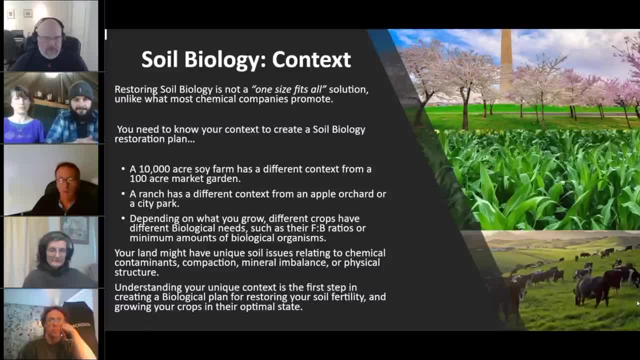 all solution, unlike what most chemical companies promote. So one of the things that has been a real benefit for what we do is that you know, no matter what kind of crop system we're working with, the foundation of what we're learning with the Soil Food Web works on everything that's out. 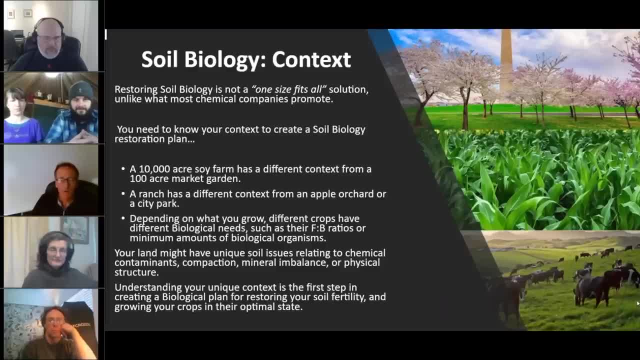 there on this planet, in the soil. You know from you know we do a lot of work with ornamentals, trees and shrubs and landscapes, to working out in large pastures and corn and soy. You know we've been very successful with the core foundation of what the course. 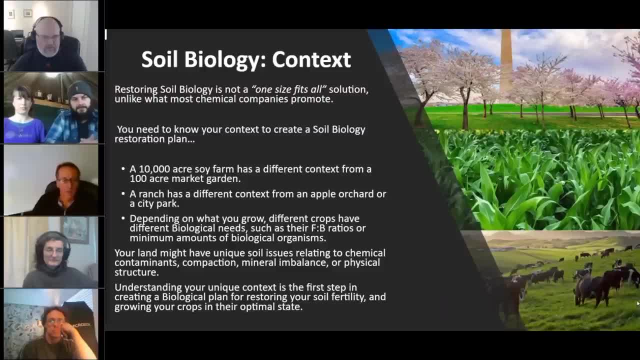 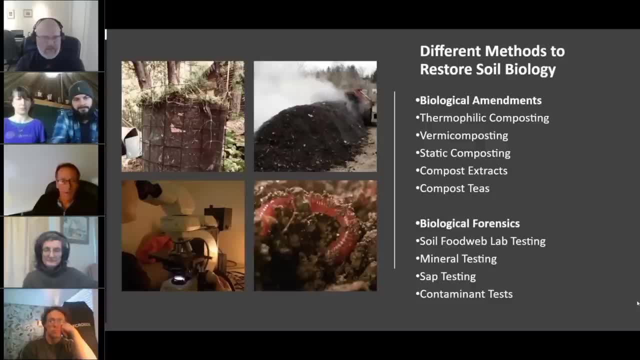 teaches us. So if you want to go to the next one, So you know, one of the foundations of what we do is actually making the bio-complete compost and bio-complete extracts and bio-complete activated compost, teased liquids, And there's many different methods to make that material. 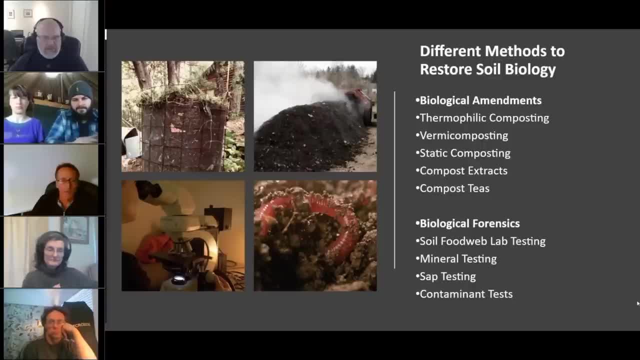 From the thermophilic compost to vermicompost, using a mesophilic process to static compost. So there's many different methods that we use to make these materials And we apply them both in a solid or a granular or a liquid, And you know one of the things that is important in making this. 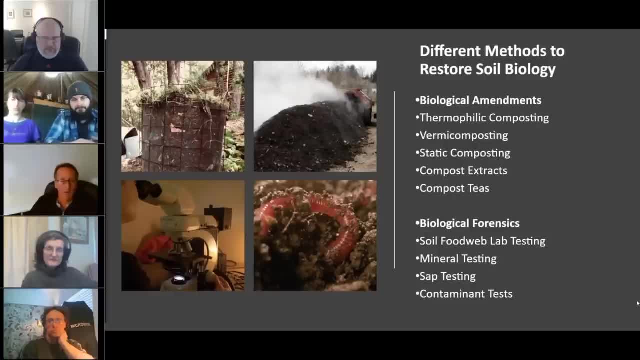 high-quality bio-complete material is doing the forensics, looking at this material and making sure it is a high-quality material, And so you know we do a lot of work with that And you know that's why we have these high standards of high-quality, biologically speaking. Next, 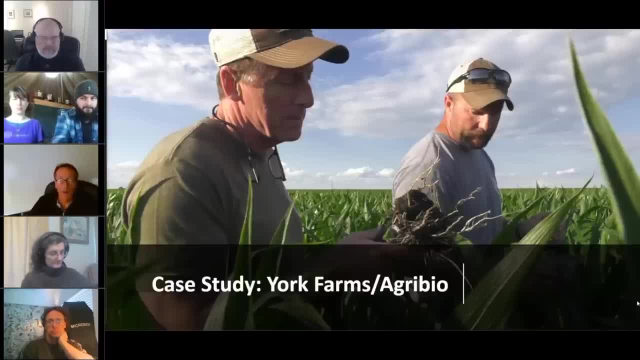 So I'm just gonna go over one of many of the projects that I had the opportunity to work on. This is one of my larger projects out in the midwest, in Jacksonville, Illinois, I met a group of farmers. basically these two gentlemen that I met, Adam York and Brad Holbrook, are the fifth. 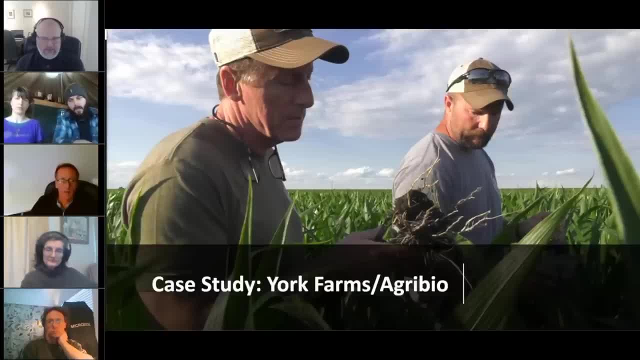 generation farmers from this operation. their, their families have been in the business of growing corn and soy for generations and they were at the point where they could not produce any more yields with conventional system or using the conventional wisdom. so they contacted me about five years ago and they were just starting to. 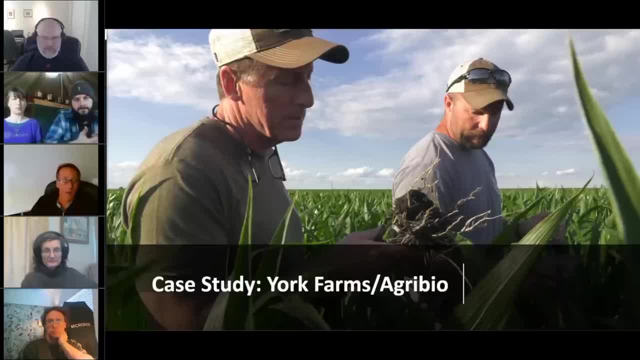 dabble with soil biology, and so I came to them as a consultant and we started this path of doing regenerative, organic and biological farming and they've been extremely successful and it's also been a real learning process for me to have or see how we can take working with small farms and take 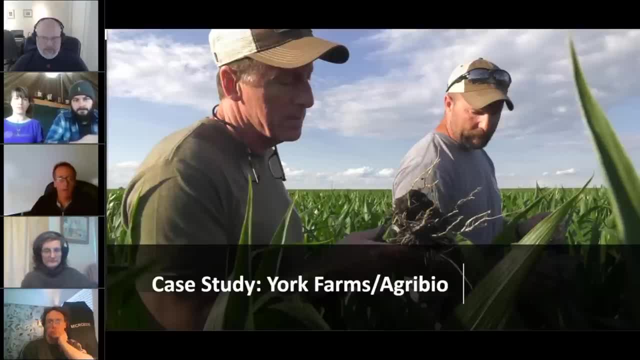 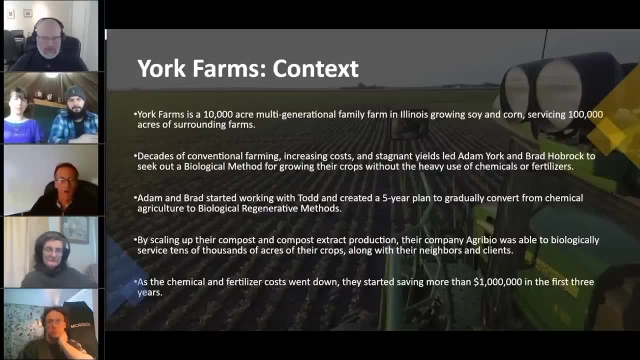 it to the next level with big AG next. so York farm. so York farm in particular is one of probably we're up to about a hundred and fifty thousand acres now with our farmland and we're working with processing our program with agribio and one of the owners of agribio has his own farm. so these two 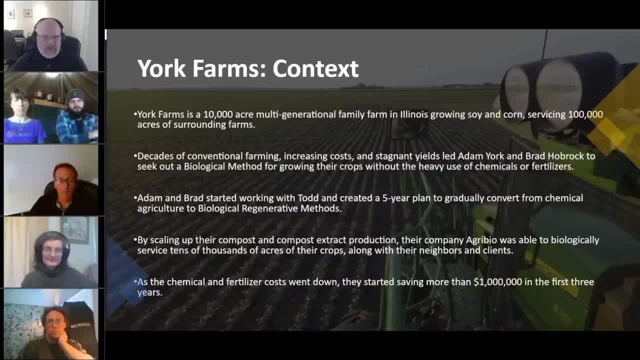 gentlemen, not only do they own and operate a facility or a company that manufactures product and biologicals, including the compost or the biocomplete compost and biocomplete compost teas, is they actually are doing the work. they actually have their own fields in their own farms, so it's 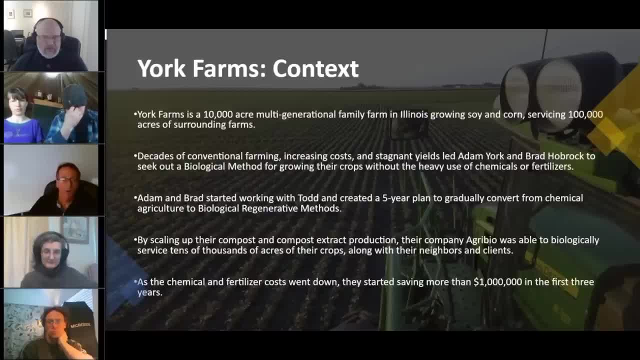 actually products that are made by the farmers, and they actually produce their own fields and their own farms, so it's actually products that are made by and used for farmers. so they personally. each one of them has over 10,000 acres of soy and corn, and 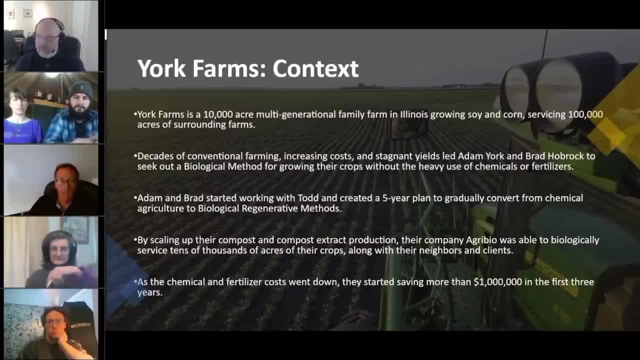 they've been, you know, in the business for four decades but in just the last five years they've been really motivated and moving forward with regenerative farming and basically what we call transitioning from the conventional system to the regenerative process. and again, you know this is a great opportunity for me to be a part of this process, and I think it's a great opportunity for me to be a part of this process. and I think it's a great opportunity for me to be a part of this process and I think it's a great opportunity for. 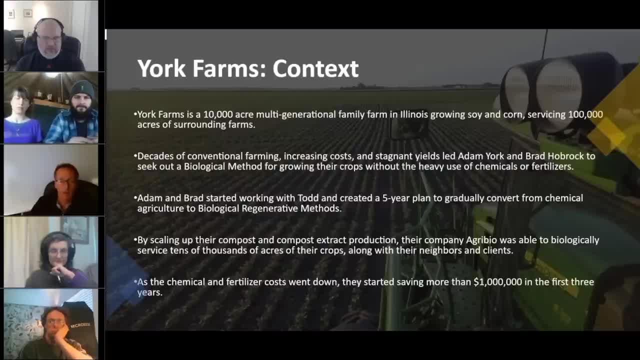 me to take what I've learned in the last two decades and really scale it up. you know we're, like I said, we're over a hundred thousand acres with our program, our process of making biocomplete compost and biocomplete compost extracts and active teas. so it's been a really 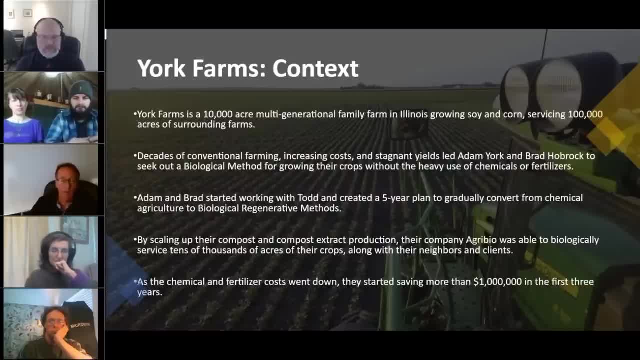 exciting project for me and also for them, because they've been very successful, and one of the things that I know, the take-home message here, is that you know, we put together a plan early on, when I first met these folks, and we put together a three and a. 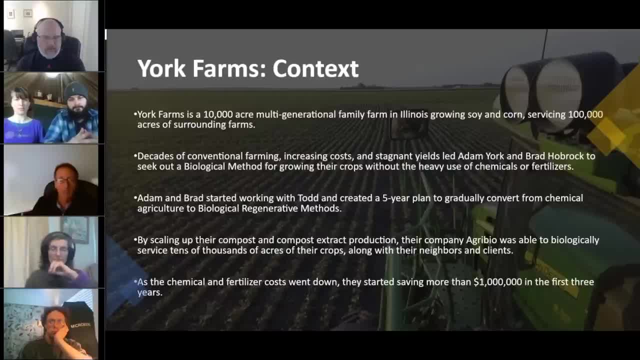 five-year program and they stuck to it and they didn't deviate from the program. that's one of the challenges a lot of folks is: they tend to deviate and do a little this and do a little that and you know they. they feel that you know this. 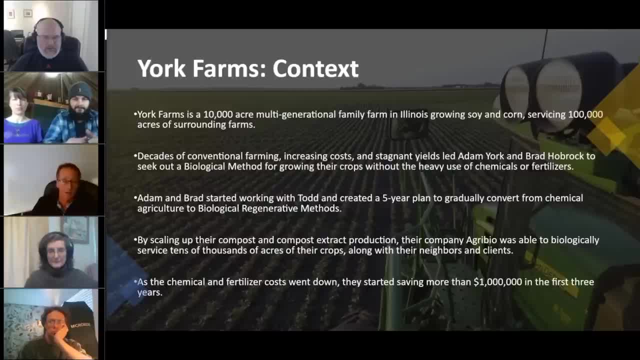 combination of work- working with conventional processes is in the work with biology- will work together. not, it doesn't always work together, but there is a process to transition when we're going from conventional to the biological regenerative process. but just within the first three years of working with these folks they saved over a million dollars just by cutting back. 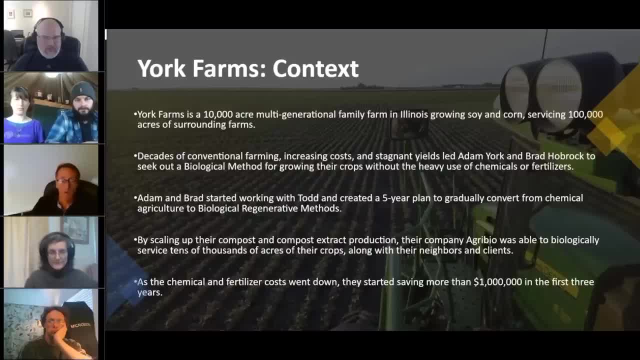 on synthetic fertilizers, going from 200 units of nitrogen per acre down to 150, to even 50 units of nitrogen, with the same, if not a better, yield, which is really exciting to see. them do that using the biological process, and so you know, some of the other things is roundup. they were a hundred percent. 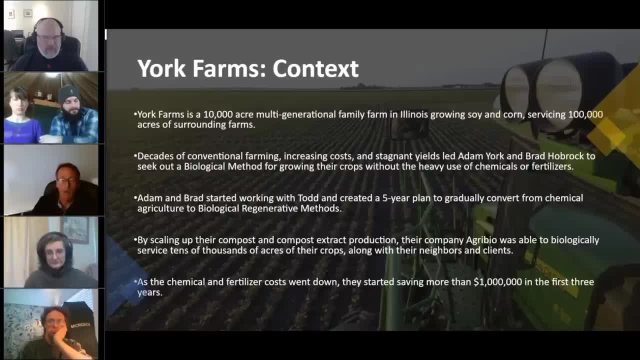 using GMO corn and soy and a hundred percent roundup. two were on year five now and they eliminated roundup a hundred percent now and they went from 100% GMO crops to there about 80% non GMO now. so really the next step is most of the even. 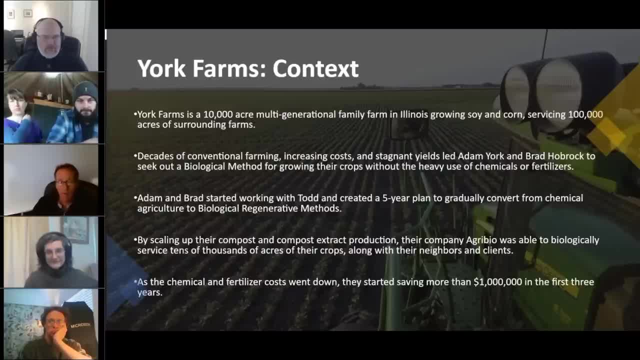 the non GMO seed. it's still coated, believe it or not. the seed is still coated with insecticides and fungicide, even though it's not gmo. so it's very difficult for them to even- you know- find these non-gmo, non-pesticide coated uh seeds. but you know, now we're starting. 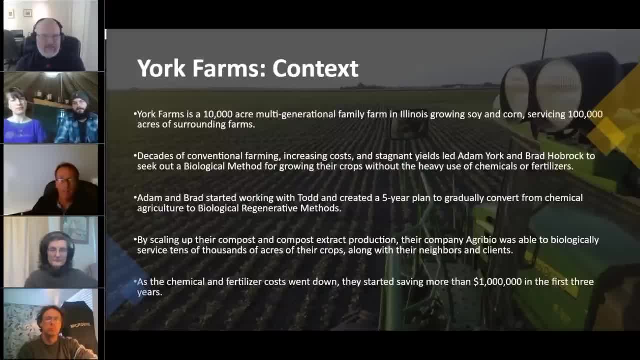 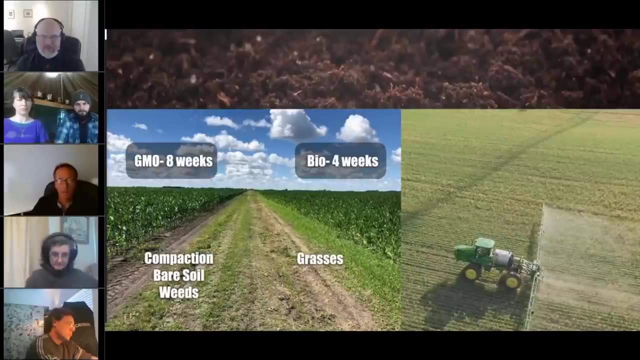 to do that. we're in our fifth year and they're actually going with what's called naked seed non-gmo, with our regenerative program, and so i'm really excited to get to that next step with them next. so you know one of the things that, as practitioners, you know a lot of us work out. 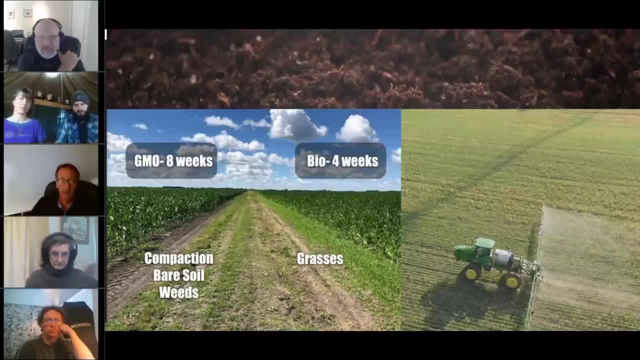 in the field. i, i personally, need to outside. i have a hard time being in the office for more than an hour or two and i get all giddy and i gotta get outside. so again i i had not only the opportunity, but the the the advantage of being out in the field a lot, and- and that's one thing i really 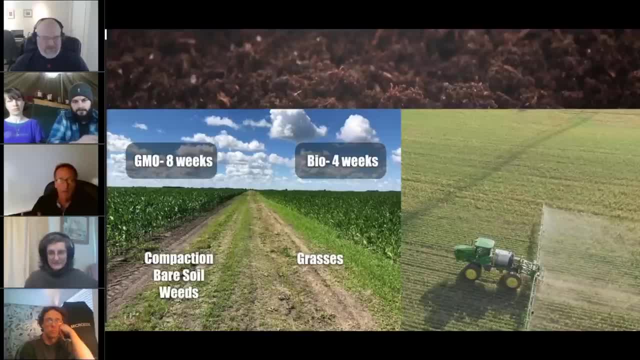 enjoy. but as practitioners- and have been in the industry for so many years is well, i noticed a lot of the little things that most people don't even notice that are underneath your feet and in this particular picture on the left-hand side, this was just this past summer, um. on the left-hand side is a conventional um neighbor who's growing. 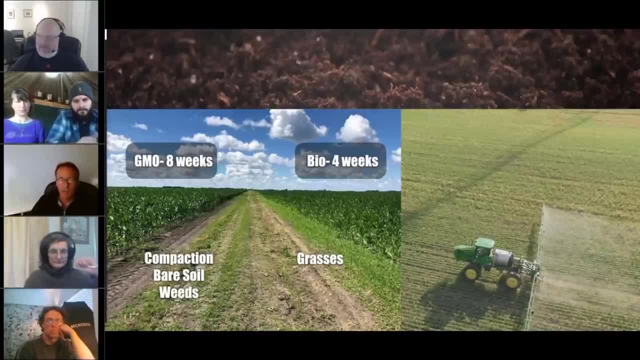 conventional corn, and on the right side is the- uh, that's actually your farms field and they're actually, uh, you know, that's a hundred percent non-gmo, no roundup at all, and even the weeds, one of the things that they have noticed quite a bit, especially within the 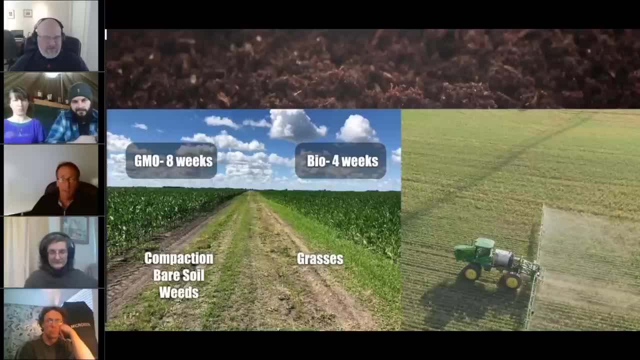 last two years is the weed species are changing dramatically from very invasive broadleaf type weeds to much less invasive grass species, and that's one of the things i noticed here is that you'll see a lot of the grasses along the edges of their fields that have been, you know that are. 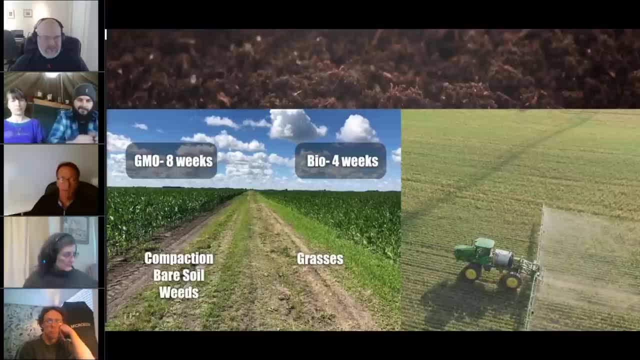 now being managed regeneratively and all the conventional fields. the weeds are very clean but you know they're still sporadic weeds throughout a lot of the conventional fields because they just can't kill every single thing. and all the conventional fields. you know we had a penetronometer. they were obviously not only very compacted but i noticed 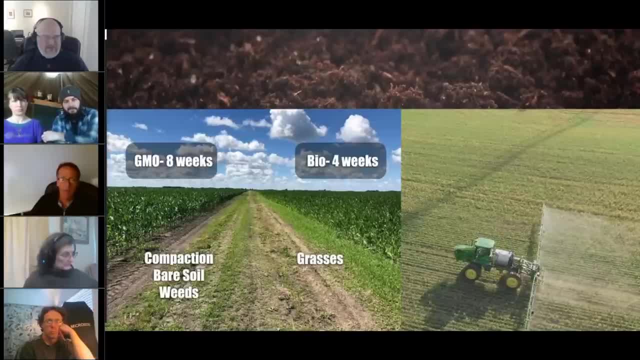 a lot of broadleaf weeds in their fields, many different varieties, where their fields, which they weren't using any herbicides, had very few, if any, broadleaf weeds. and a lot of these, uh less species, when you look at their biological relationship, their fungal to bacterial ratio. 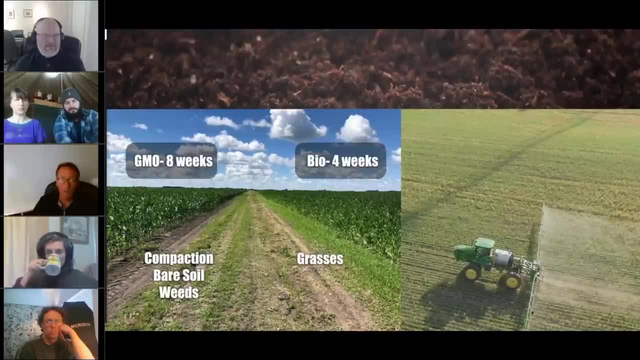 grasses are much like corn versus the broadleafs are much different and the field on the right is actually us spraying. this is uh. they actually invested in a sprayer just for applying biologicals, the liquid bio complete compost, the extracts and the actives, so i was really excited to 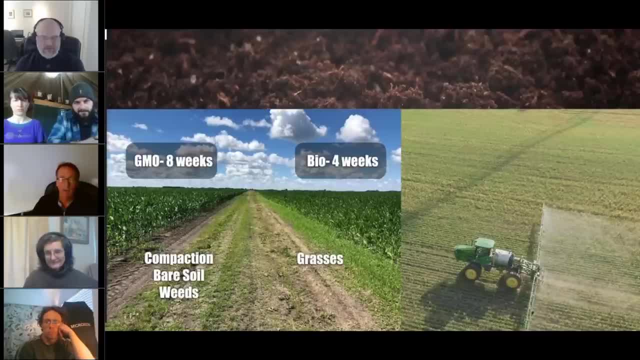 find out, they actually made that move financially, which was a big one, because these, these rigs are a quarter million dollars, um, specifically just to apply the liquids. this past season, present years, they were. actually we were trying to use their conventional sprayers that had all kinds of herbicides in them. it is very difficult to, to you know, clean them out and try to use. 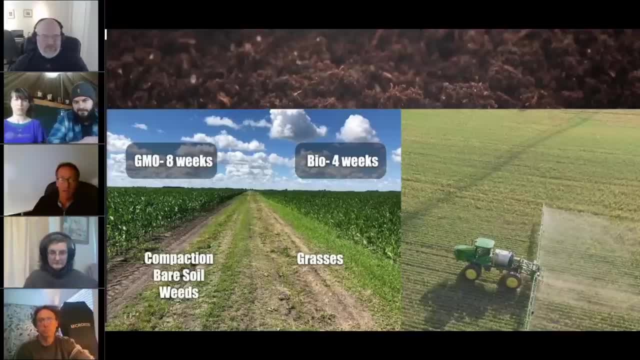 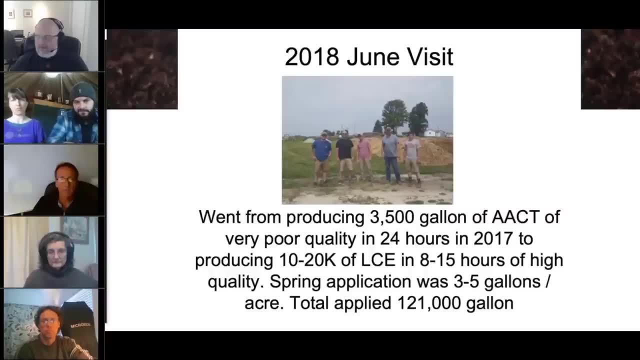 biologicals. there's just too much contamination, so that's actually us spraying that exact same field that you see on the left. so you want to go to the next slide, please? so this is in june. this was my june. i usually visit these folks two or three times a year, and i started back in 2016 or 17, so this is. 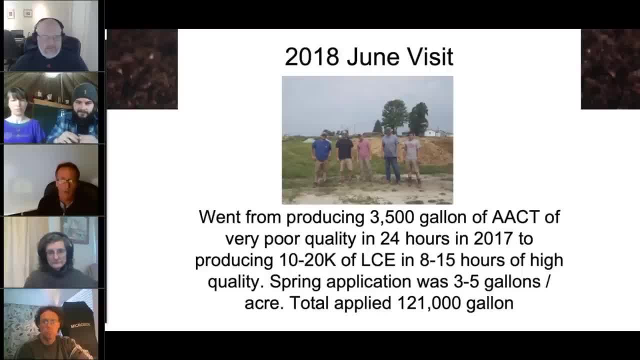 our june visit. so just in one year, from 17 to 18, we went from producing 3 500 gallons of activated aerated compost tea and, and i have to say it wasn't a very good quality. it was basically they were making excellent brown water, but they were getting results from it, and so 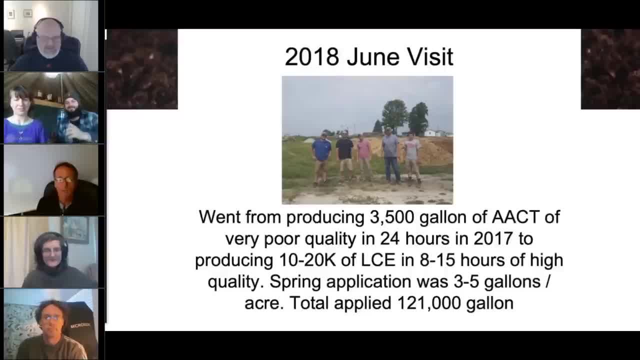 after getting all the data, we what we realized? that the reason for the results that you know they were getting some improvements was mostly because of the foods and the amendments they were applying. it wasn't the biology. how did we know we were testing? we did we? you know every single project. 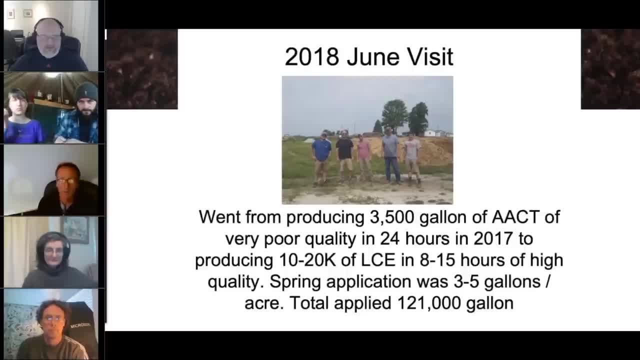 i go on. we bring our microscopes, we bring our pipettes, we bring our slides, and so we are able to test on site, which is, you know, a real benefit and advantage for a lot of us, because when you send samples, there are some challenges, uh, you know, with sending live samples. so, um, in general though, 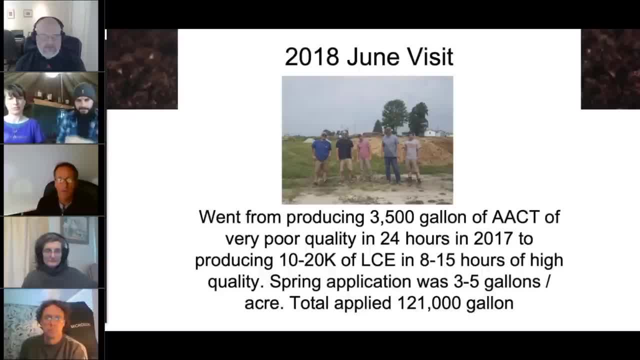 um, you know, they, uh, they were. they had seven 500 gallon brewers that they were basically making active compost teas, which you know, in our world- i think elaine coined this quite well- is it was really putrefied liquid, uh, compost teas. it wasn't really. you know what we call vial complete activated. 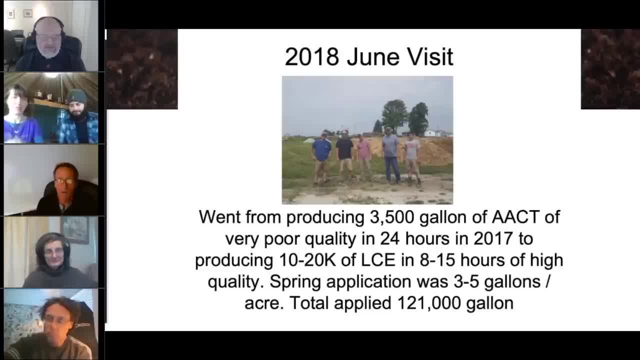 by any means so in a 24-hour period. they were making a scale of one to ten, probably about four when it comes to bio complete active compost teas, and so in 2018, we went from making compost teas to top of extracts, because one of the challenges when you start to scale this up, you run into a lot of 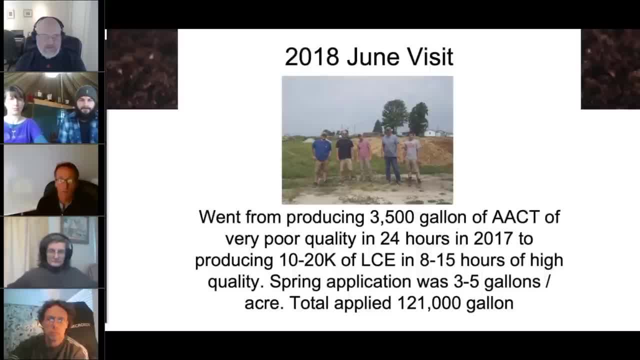 challenges when it comes to time and volume, and so we had to produce up to a hundred thousand gallons of compost tea. and so we had to produce up to a hundred thousand gallons of compost tea. and you can see that the different amounts of compost tea and the different amounts of compost tea. 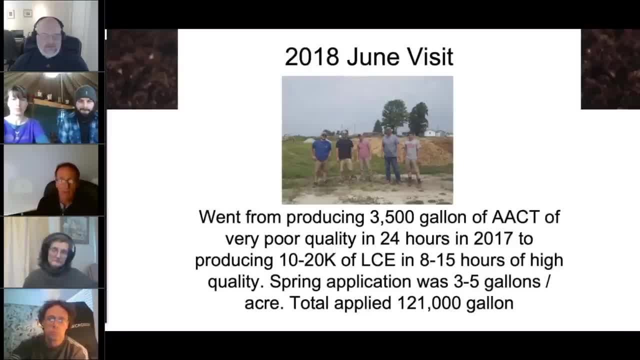 and the different amounts of compost tea have a very different composition. now that becomes really challenging when you start trying to make that kind of active material. so to simplify things, which you know, maybe at another time we can talk about the difference between active tea or active compost tea versus just compost extract. but anyhow, going forward, we went and set them up with a compost extractor. 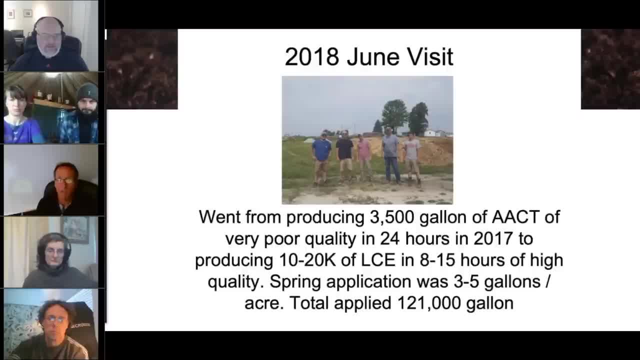 able to produce between 20 and thousand gallons of liquid compost extract. that's what the LCE is in 8 to 15 hours, of much higher quality. we were really excited about the numbers we were seeing under the microscope just with an extract, so there was a big difference. so the spring application with the compost extractor. 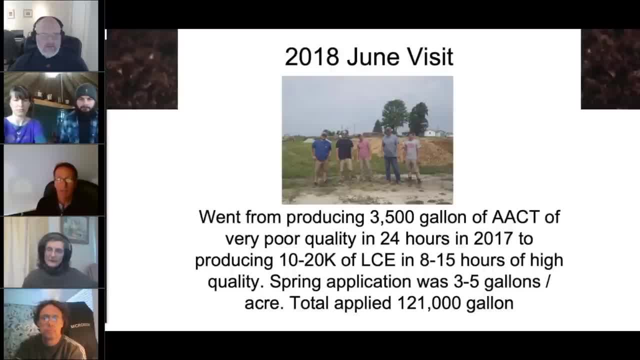 we were producing 10,000 plus gallons a day. we were applying it only at three to five gallons an acre, which I know is really a low rate, but we were doing it in furrow, so that real good quality compost extract was being applied directly to the seed in furrow in the springtime, and that was that first. 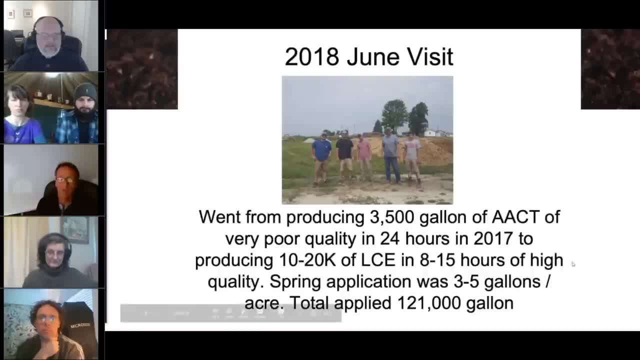 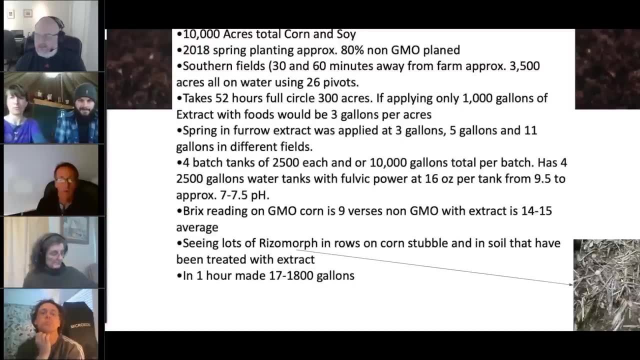 application was 121,000 gallons and that was just for the 10,000 gallon operation. it doesn't include all the other acres that we did. you want to move to the next one, please? so, anyways, this is just some numbers you know to show you what we did in 2018, but again, this was a 10,000. 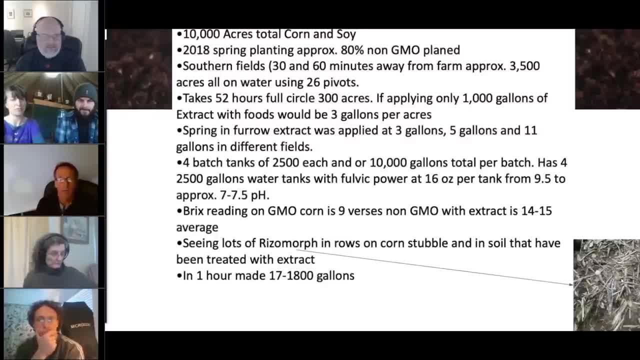 acres of corn and soy and so 80% was non-gmo. they also, out of the 10,000 acres, they have about 3,500 acres about an hour south from their, their main farms, and it's a very sand- they call it sugar sand- but a hundred percent dependent on. 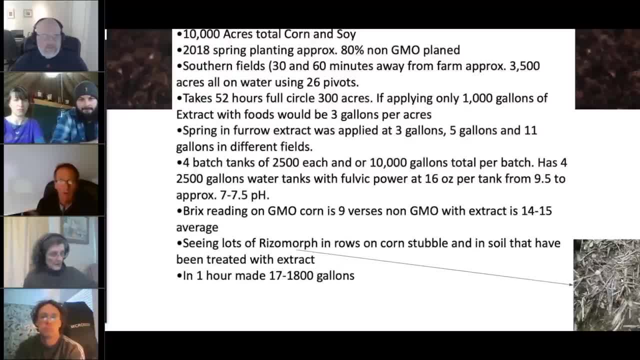 irrigation, unfortunately, so they had about 28 kibbutz. there is sorry 26 pivots that managed the 3,500 acres down south, and so I had the opportunity to go down there and we were actually- I was actually there when we were doing the injection, and so one of the methods that we were using to 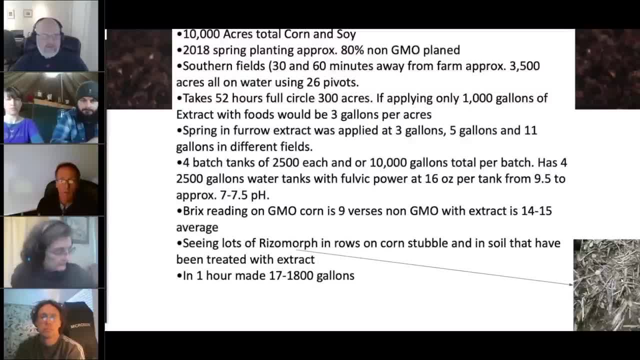 apply. the compost extract was through pivots. so down south the 26 pivots each got this compost extract. but what we did is we took the compost extract and then we put it into a bin to make the compost extract. but what we did is we took the compost extract and then we put it into a bin to make the compost extract. 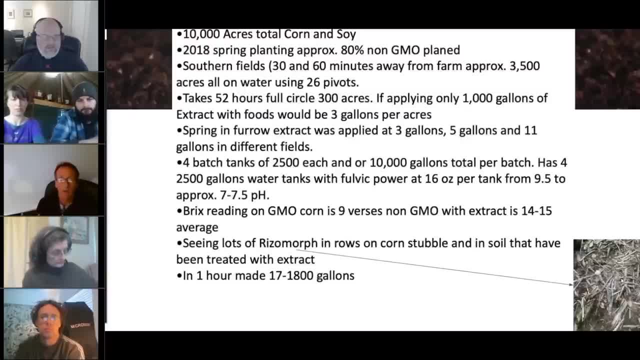 extract and we put it into these brewers that they had. so we were no longer using these 500 gallon brewers on site to make the extract. and so what we did? we converted them, we put them on trailers and then we would basically download our compost extract into the pivots and then, and then apply the foods and aerate and 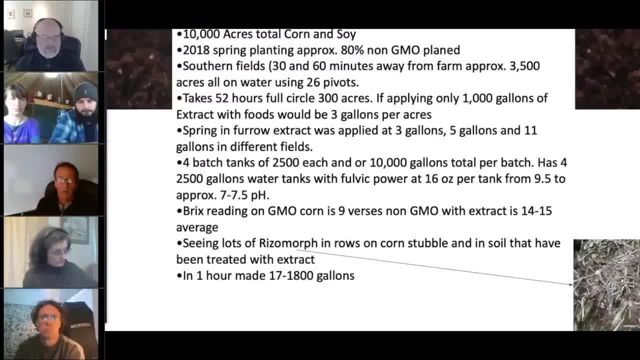 then inject it into the pivots. so you know it's not a lot of product, but we were still really effective at getting the biology out. so in a 52 hour full circle we covered 300 acres and we applied about a thousand gallons of extract with foods, which came out to about three gallons per acre. so again, 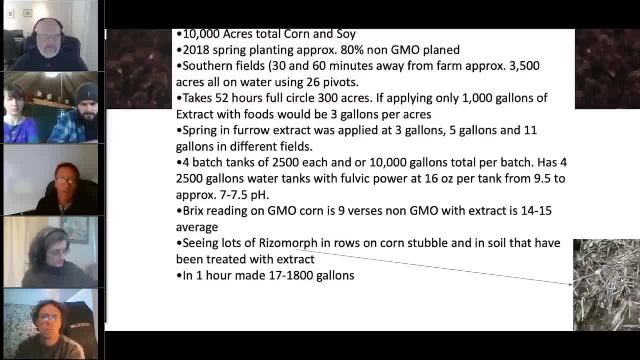 it's not a lot, but it is of high quality and we did see really good results with it. so, moving forward, we started experimenting with the three gallon, five gallon and 11 gallons, and what was interesting is that sweet spot was around five gallons an acre, so even at 11 gallons we didn't see that much more of an. 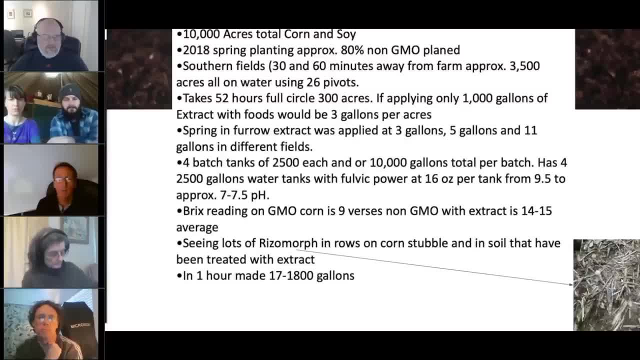 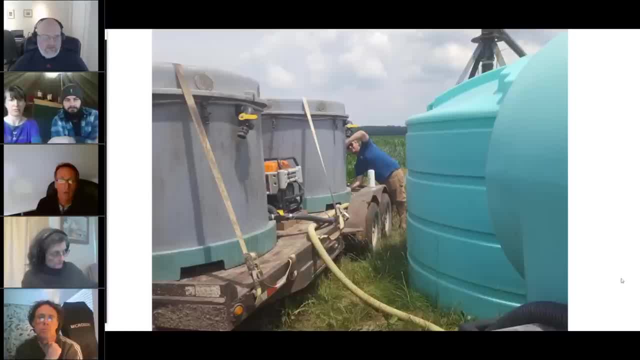 improvement than we did with five gallons, but we did see an improvement with five gallons versus the three gallons. so i'm just going to show you in the next slide basically how we applied this out in the fields. so there we are. so these are the 500 gallon brewers that they originally started. 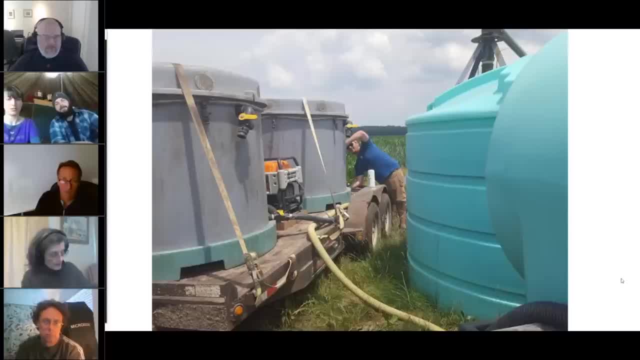 using- and you know it was really challenging uh for these folks to do- seven 500 gallon tea brewers, put it out and then make another uh batch with the seven 500 gallon rows, which is 3500 gallons. so we were really limited by time uh in volume. but one of the other big, big challenges as 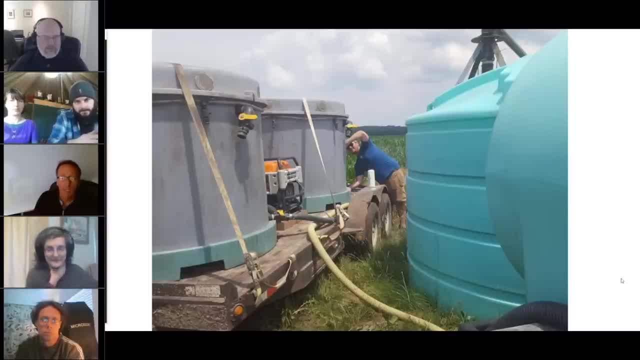 everyone on this call knows, especially elaine, is that cleaning and disinfecting 3500 gallons is not an easy task by any means. it took hours, if not days, to clean those tanks, especially if you're not good about cleaning them out directly after application, because then 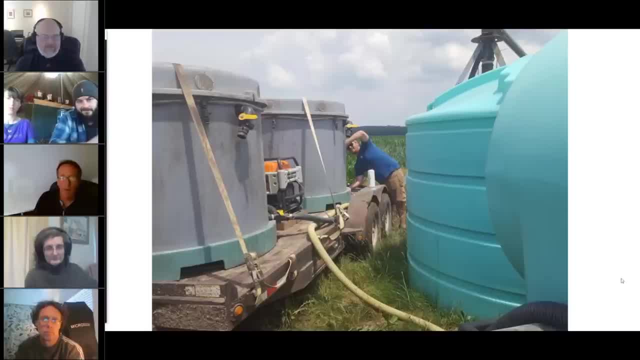 it's like you know paint trying to get paint off on the wall. so, anyhow, we figured out systems and that's another really important thing you scale up like this is quality control. so we had methods and systems where we made sure, because these tanks that you're looking at on the trailers- 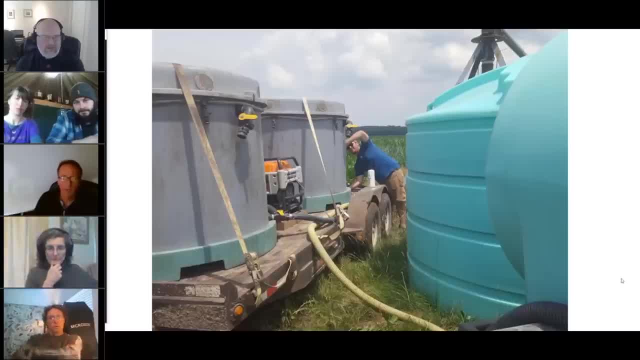 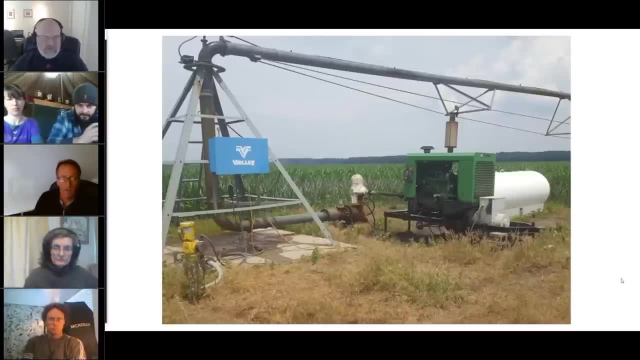 but when you're working with trucks and they're being used in the Tatooine to work with you, they're maybe so much better. so we're also going to show you some other projects that we're doing that have been able to make real-time cleanートil for the 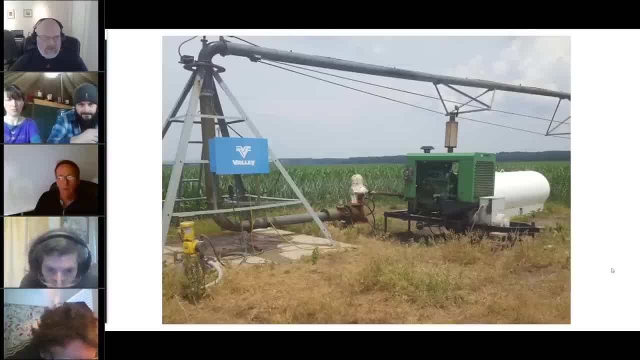 tank and these are again bigger than the one we had in the past and they're kind of an hour of clean. some are actually gas. this is a big diesel motor that's driving this pivot, but you know they have a combination of motor: diesel motors and also electric. 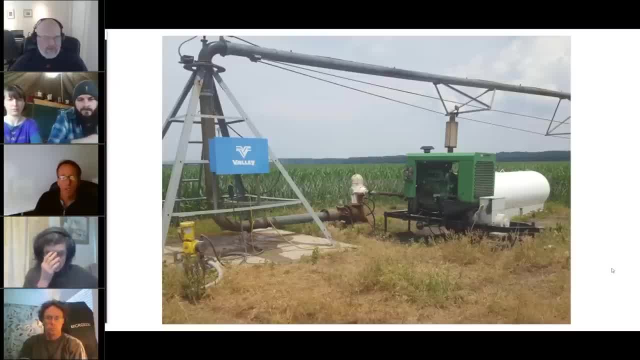 but anyways. so this is where we were actually injecting a thousand gallons of activated extract into this pivot again. it took about 52 hours and one full circle to cover 50, to cover the 300 acres. excuse me, but we had really good results with it, just at that rate because it was tested. that's how we knew. 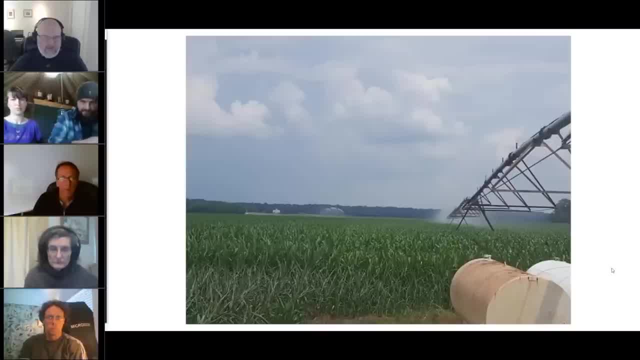 and so you want to move to the next one. so again, here's the pivots going out. you'll see one in the floor that's actually the same hit it on the foreground. so this is a big monster. so very high, intense maintenance to maintain these things. but what a great way to apply the bioactive activated. 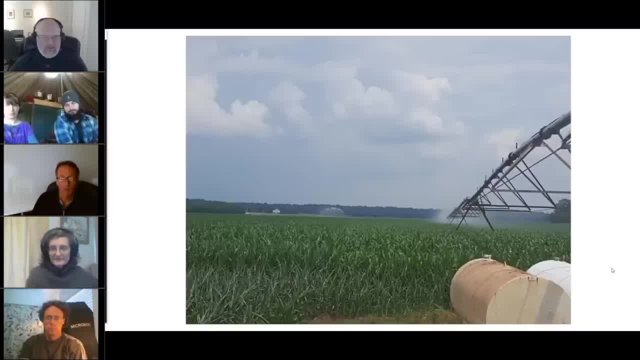 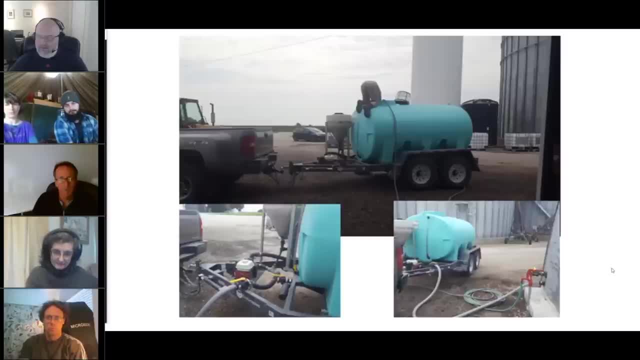 compost extract, and so you know, very effective method of applying the biology if you want to move to the next one. so another challenge we had is how do we move all this biology to each pivot? so we went from the cumbersome tanks which we you know, the cool thing about it is that we took these tanks or not, that we were no. 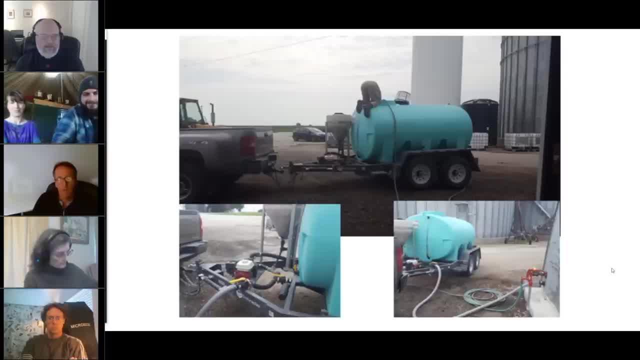 longer using- I mean the Brewers- and we converted them and made them. so we did, you know, least eight the material right there on site. so we went from that to these pony tanks. this is actually one of the smaller pony tanks, but we have 500 and thousand. 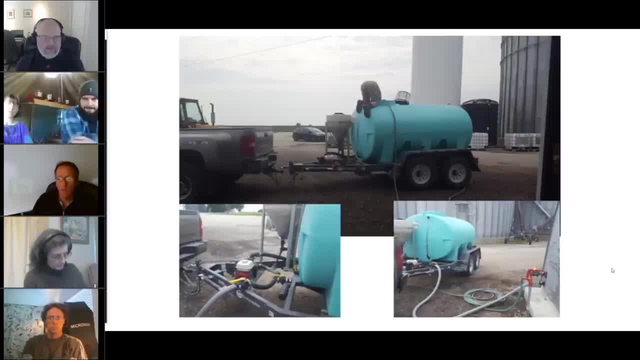 gallon pony tanks and these tanks actually allow us to transport and deliver the extract. and again, this isn't an activated tea, this is just a extracted- you know extract from high quality of vermicompost that they actually make on site and that little cone bottom tank and to the left of that, 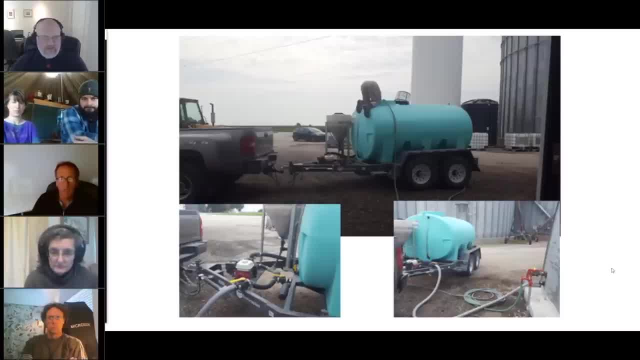 tank is actually all the foods, things like fish, the humates, the molasses, and we have our own, you know, special recipes that we've kind of developed for these guys. but that allows us to inject the foods directly into the extract and either either activate, because those tanks have aerators in them, or we'll just inject. 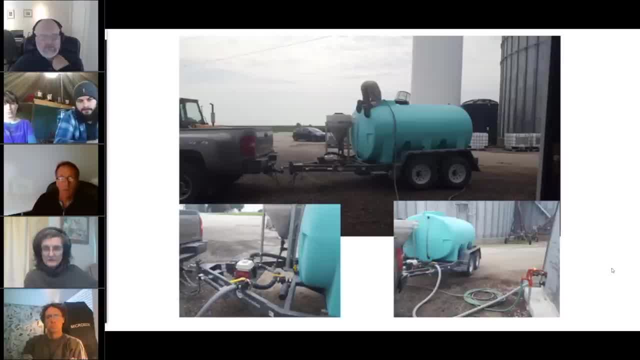 those foods into the tanks and put them right out right away. you know, because when you might be using, let's say, more than five gallons of fish per per gallon, per, let's say per five gallons, per thousand gallons, you could actually add too much food and it'll go south on you. so you might have to activate it. but this was a 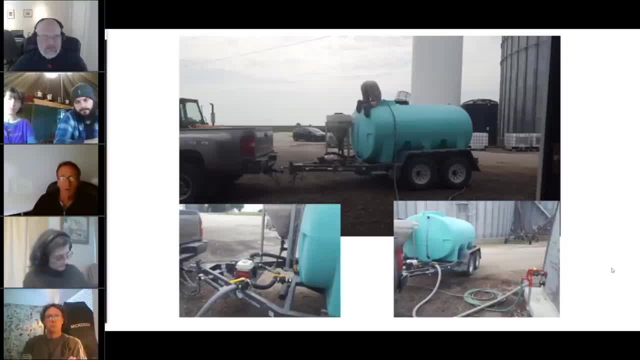 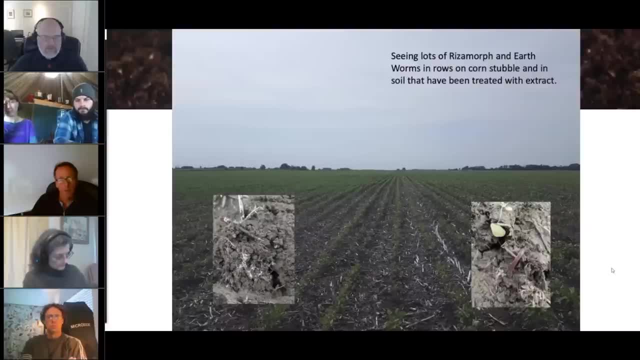 great process to us, for us to transport large volumes of extract and then activate it there, right on site, with the foods, if you want to move to the next one. so anyways, you know some of the the results were. you know, not only did we see really good results on the microscope, but also visually, and that's one of the 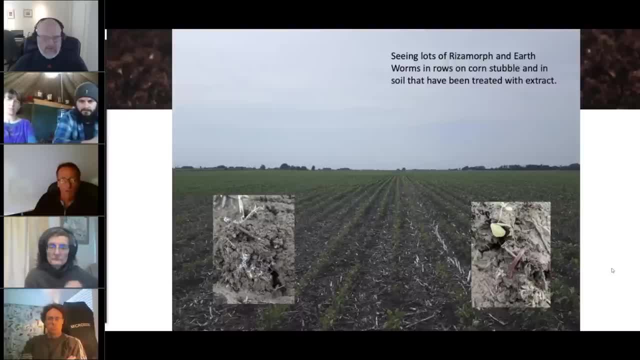 things as a practitioner that you want to kind of zoom in on or zone in on is: look at things underneath your feet, look at what's happening, and one of the things that these folks notice is the rhizomorphs everywhere. they never had this before. when I started with them, there was no fungi at all on the top of 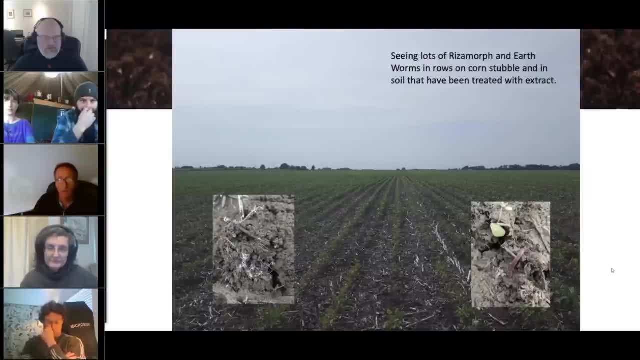 the soils or in the corn stalks, in the stovers, in the residual, and they also had no earthworms. well, guess what? we have lots of earthworms now and we have lots of rhizomorphs, and they also noticed in the in the residual, especially with the corn stalks. 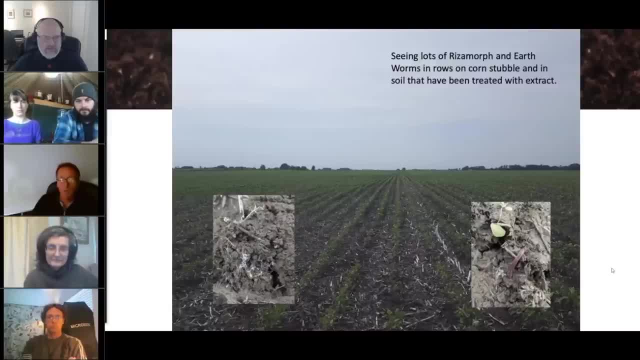 is there's a completely different hue. when you're looking at these fields from the roads, you can see a completely different hue on their fields compared to the conventional arms- a big difference. so it's really cool to see that visual. and I was just there about a month ago and same thing. you know, it's just I'm. 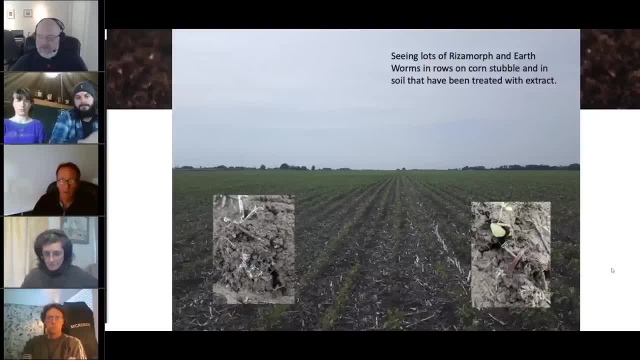 seeing the beautiful rhizomorphs everywhere on the corn stalks and that are still sitting there on the field and they're getting really good results ground and i'm seeing we're seeing lots of earthworms and i'm seeing lots of weeds- non-invasive. 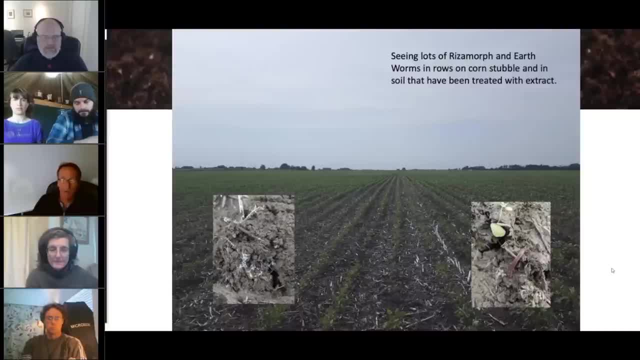 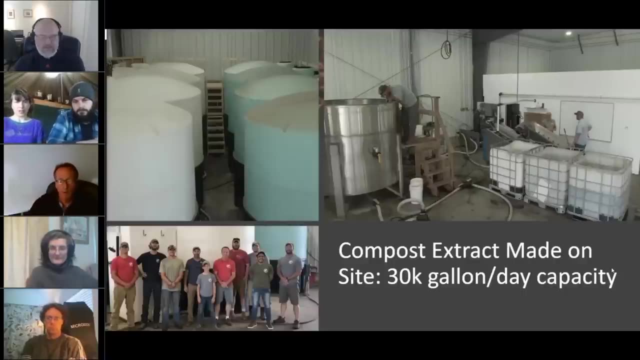 weeds that they never had before, uh, these, these perennial prostrate type weeds that are non-invasive or competitive with the corn, and that's something they never had before. so really cool stuff next. so, anyways, we went from a big hoop house, uh that we started with building. there's a steel building. 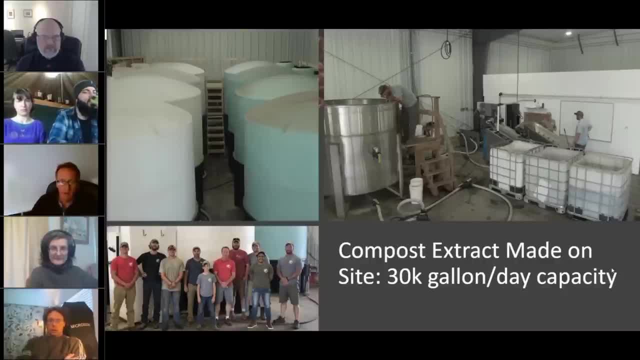 but it was like a hoop building uh to a state-of-the-art uh extract compost tea center. you know it's close to a million dollars this building, but man did they do a great job at setting it up. but anyways, the the photo to the left, you'll see the the batch tank to the right, 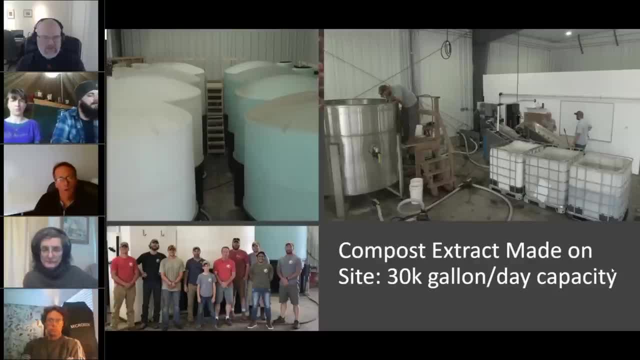 and there's basically four, ten uh four uh 2 500 gallon water tanks and a lot goes into the water. we are actually structuring the water, we are dechlorinating the water. so there's two ten thousand gallon tanks outside before they go into the water tank sources that we're going to make. 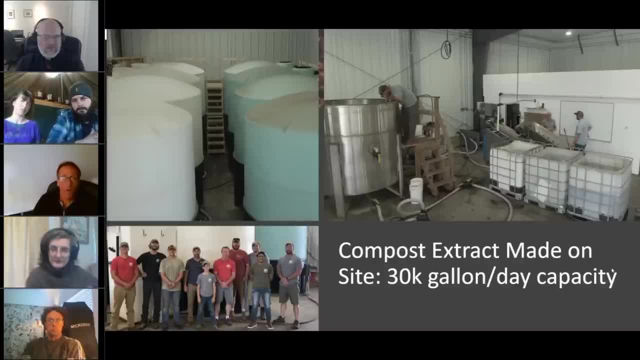 extract, um, so that's what you see on the right hand side- is four, 10, uh, 4, 2500 gallons, so that's 10 000 gallons each. those are the batch water tanks that have been basically the water's been prepped before we make extract, and on the left side, those are the batch tanks of extract once. 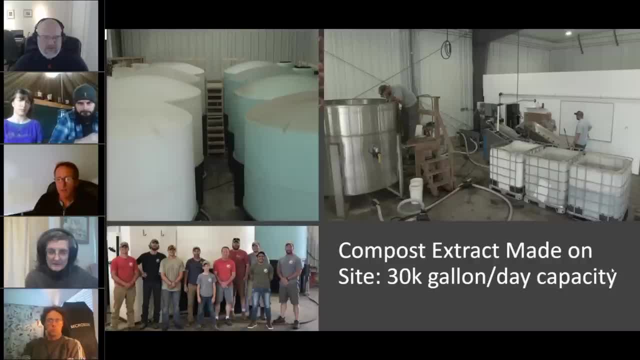 it's made, and to the right you'll see basically the extractors. this year we're going to be running two extractors, so in an hour we can make, close to you know, 5 000 gallons um. so this says compost extract made on site, 30k gallons a day capacity. so we're really really scaled up. and this is the crew to the left. 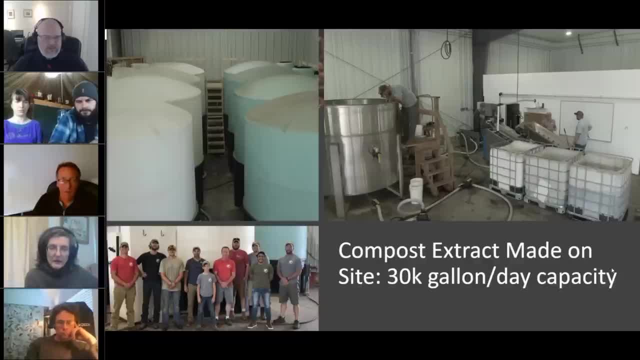 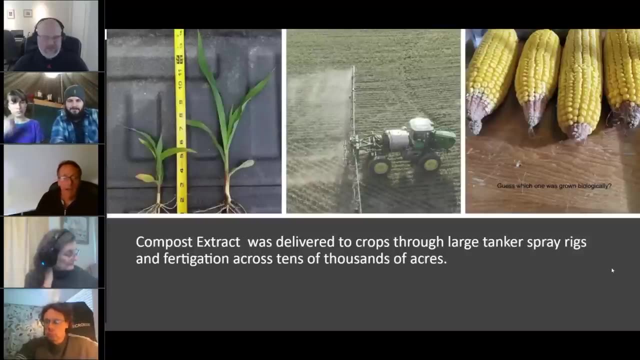 the agro bio crew, a great group of guys very, very smart, um and uh, basically we this was, uh, this was this past summer actually. um, you want to move the next one? i know my time's getting cut, but yeah, so some really exciting uh data that we're getting from this project. uh, on the left hand side. 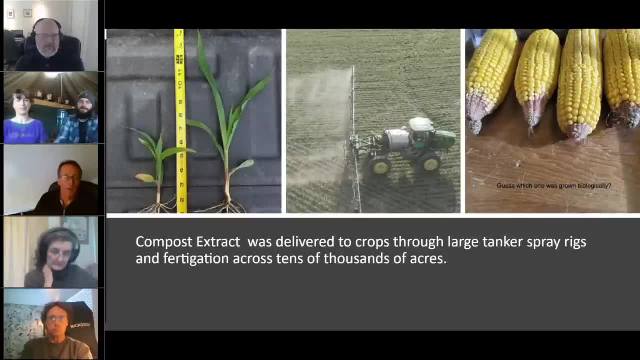 you'll just see some corn growing, uh, from a conventional corn on the left to the regenerative corn on the right, and both, uh, both corn, uh stocks that. you see that, um, that's probably a very early stage, um, but anyways, both of them have uh, one's conventional on the left, the one on the right is regenerativeYURA, which is a conventional corn, but we're all talking about corn growing up and on the rest of the list for these few years are what we're seeing: now, two or three and a half years. the next four years, we're just seeing some new plants coming out of this grid, because this big new plants 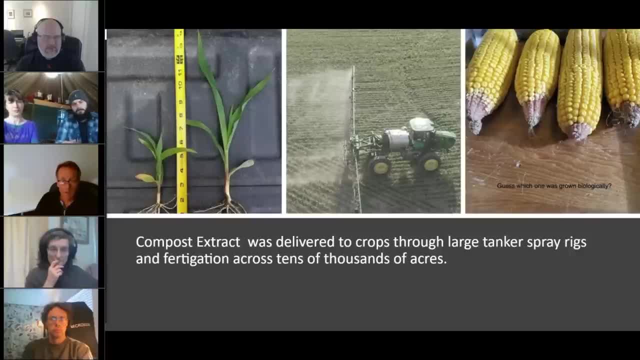 a lot of the firstlives. we're not seeing these new plants, but we're seeing these new plants that are growing up and growing out. regenerative growing, the biological program, no pesticides, no GMO corn and no roundup at all. both are getting the same amount of nitrogen. look at the 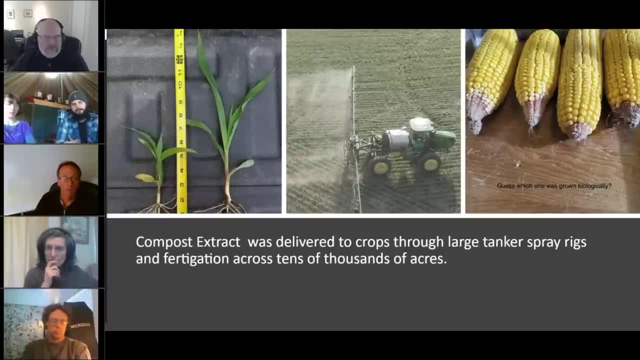 difference. so this is about 120 units of nitrogen, and yet the regenerative corn has got a much better head start than the conventional. and that's actually us spraying in the middle there with the new. well, I think it's a used sprayer, it's about a hundred and ninety feet, and we've modified it so the pumps been 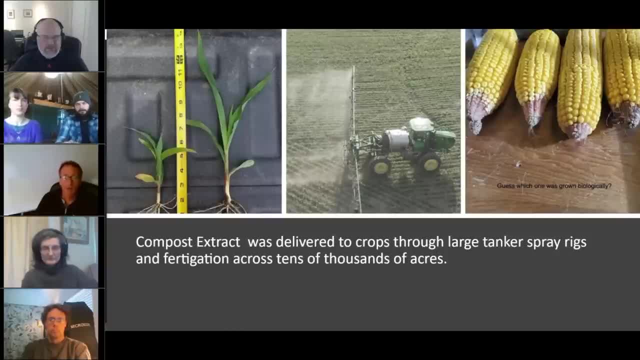 modified, the tips have been modified just to put out the bile, the bio complete compost teas, and one of the things that we've really noticed in the last two years is that the kernels and the, basically the stocks, the corn. I mean we're just seeing so many cool things, but we're starting to see the corn fill. 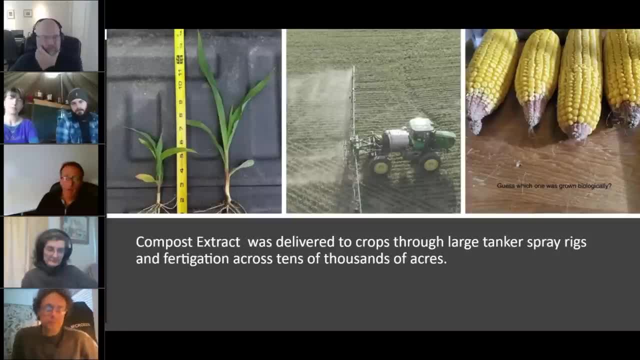 out a lot more on the tips that they've never seen that happen. you know, usually through nutrition they can get this done, but they have a hard time with it. and this is actually corn feed. but they definitely notice a big difference with the quality. the protein levels have gone up quite a bit. the bricks have gone from. 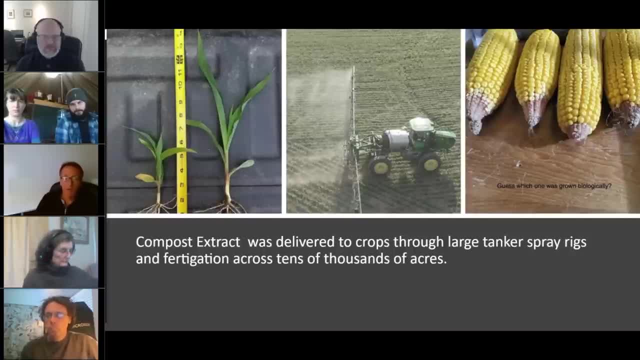 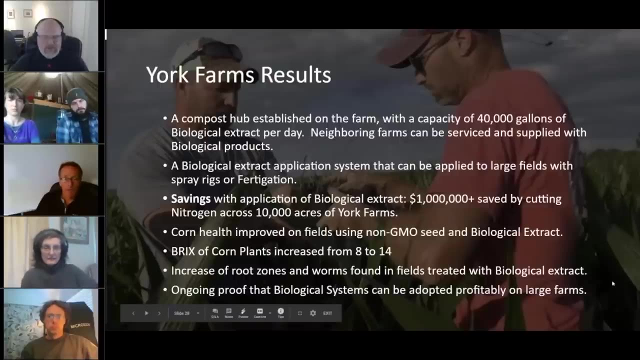 between 8 to 10 to. we're close to about 14 on the brick levels now, so we're just seeing some really really neat stuff happening. you want to go to the next one? so you know, just kind of summarize here with the York farm results. you know they. 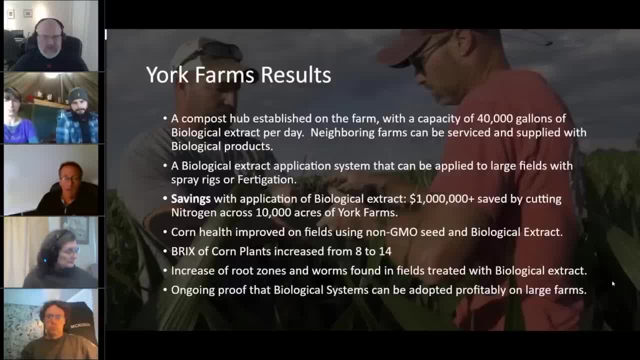 because they are becoming so successful with the regenerative process in the biological process, they actually are now becoming a hub for a lot of their neighbors that work, that are and that are becoming regenerative, because you know all their neighbors are scratching their head going. you know what is this? 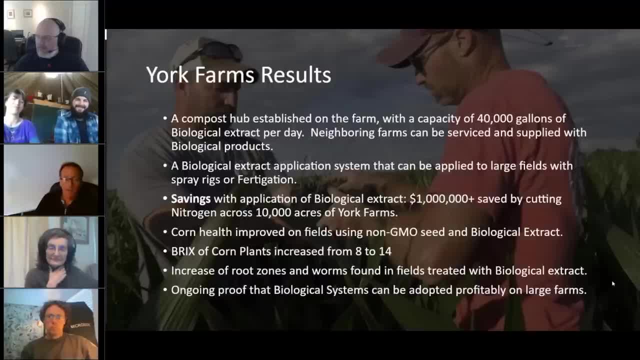 that you guys are doing, because you know everyone kind of looks at these guys, you know, thinking they're just doing some crazy stuff and wasting their time and money. but they've actually are saving money, a lot of money, and they're growing higher yields than their neighbors and they're saving thousands. 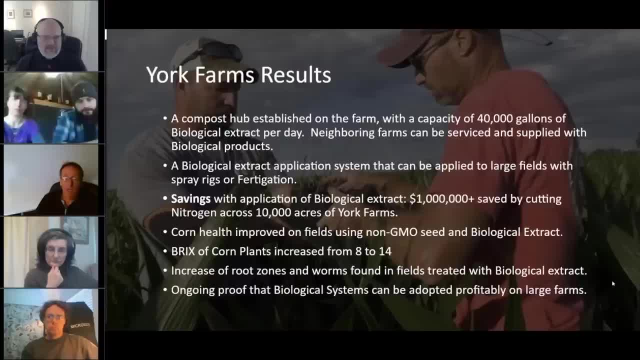 if not millions of dollars. I mean it's really exciting collectively, this whole group, you know the hundred fifty thousand acres total. I mean the savings are enormous. so the biological extract application system that can be applied to large fields with spray rigs and fertigation. so again, you know these guys. 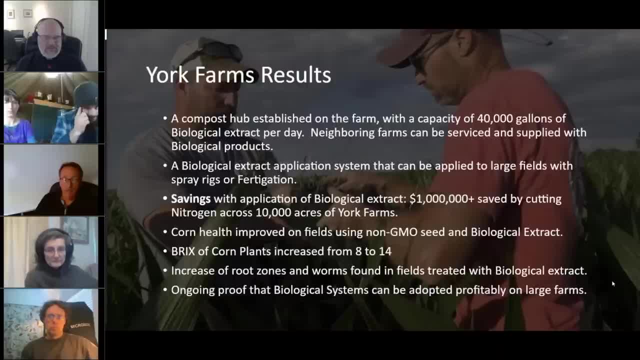 have been very successful at doing that and savings are enormous: the health of the corn, the quality of the corn, the yields. so you know they are actually making money. now, you know, typically, I think you know, you're lucky to make a hundred dollars on an acre and these, these folks have increased that to almost. 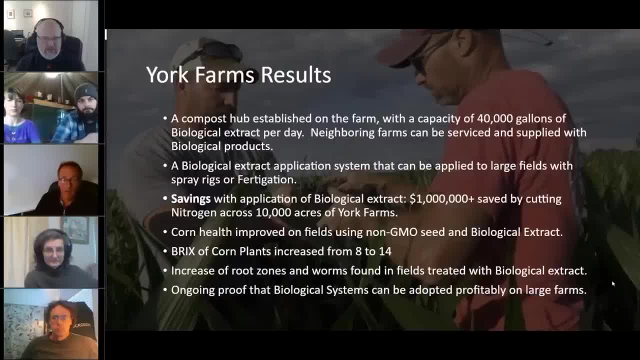 four hundred dollars an acre actually making. so they're saving an enormous amount of money and they're actually making money now. so, anyways, ongoing proof that you know the biological system can be adopted and profitable to both small and large operations. you want to move to the next one. I think this might be the last one. 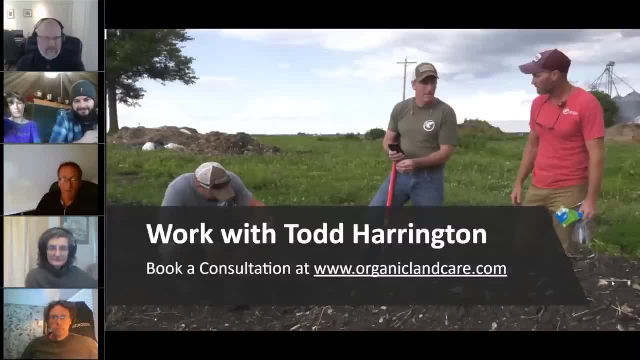 so, anyhow you know, I am consultant with. you know, the website that I have is- it's actually a fairly new website just for the consulting- which is wwworganiclandcarecom. I invite you to come and visit my site and I just want to thank everybody here for allowing me to do that. Todd, thank you. 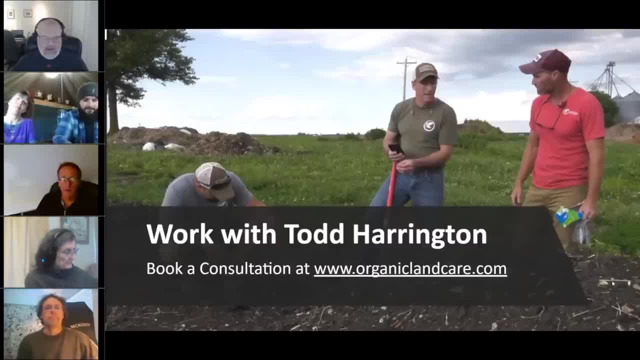 very, very much it's. it's all amazing to you know, I get folks, farmers I get in contact with, and I get this comment quite a bit which is: oh, that's great in the small scale, but it really you just can't, can't do it on a large scale and 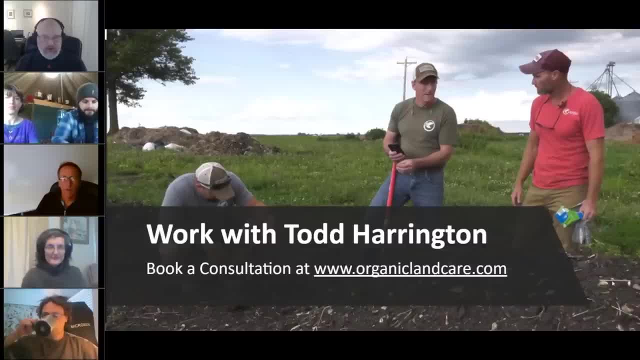 that's just absolutely not true. you can do it on a large scale. you just be mindful and you have to really think through the processes and work with your farmers to make that transition. so I give these guys a lot of credit for what they've done and what they're doing, and you know the commitment that they've made. 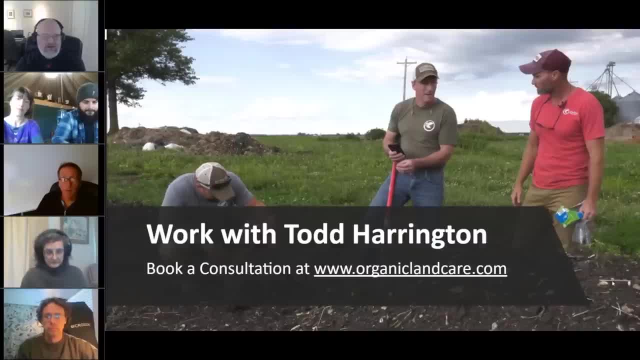 financially and time wise. you know, it's just. it's right there needs to be more of these guys out there. that's how I can agree. agreed. yeah, I have a client that's very similar to yours, that's passionate about this, is taking the forefront in our area. it's the same thing. it's amazing to watch these folks work and 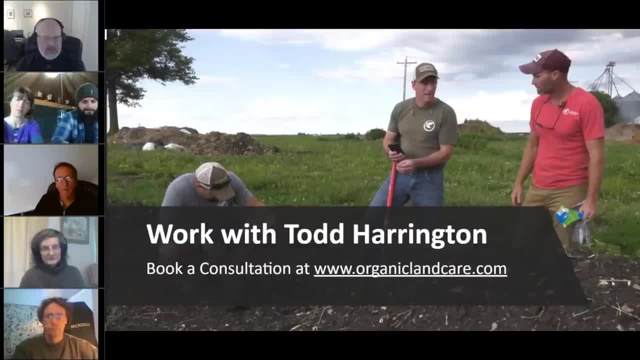 they're very good at problem-solving. you give them a challenge that I'm gonna figure it out and they do. they figure it out. so there's a lot of people getting involved in the courses. you know there's still a lot, as Elaine knows a lot of. 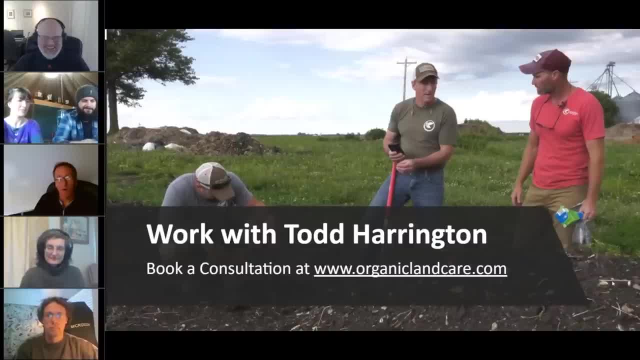 conventional farms out there and and so there's so much opportunity out there globally for us to really take this, this science, you know, and and make it the norm. it's, it's a huge paradigm shift that's occurring and it's just a huge opportunity, so many folks, to really make this change. we need to do it. 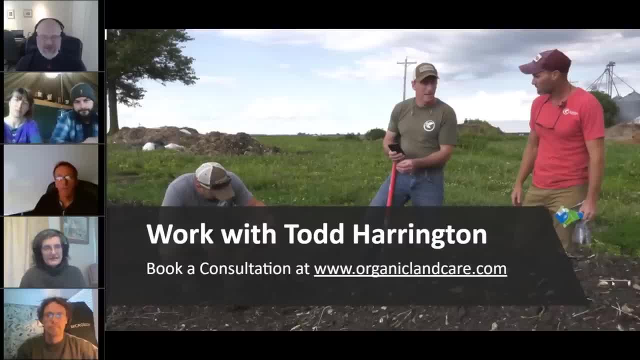 on a much larger scale. and you know we get, we get kind of overwhelmed by the cost of one of their sprayers. you know two hundred and fifty thousand dollars for just that one piece of equipment. but if you're a large-scale grower, if you've 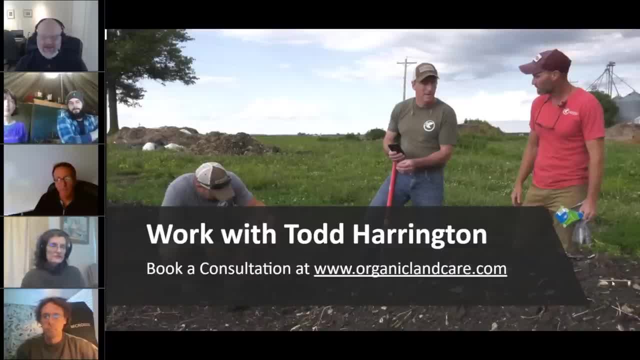 been growing on ten acres every year. you've been buying gigando size equipment for as long as you've been alive. your dad spent that much money on the tractors, your grandfather spent that much money and they don't even blink when they have to take a loan out for, you know, to a million dollars or two million dollars. 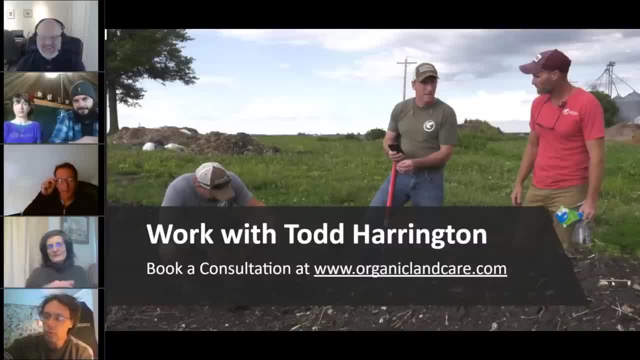 that's just what they expect, and so we have to not get unnerved by so expensive what you know what happens if there's a failure. if you're keeping track, if you're using that microscope, there won't be a failure. this is not gonna not work. so 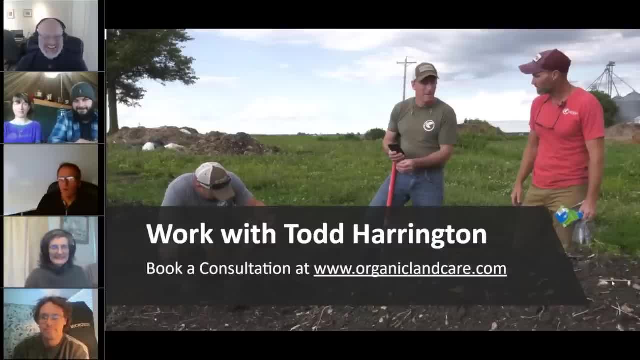 attitude. they got a couple planters. but the cool thing, Elaine, is that we have been able to down those equipment and modify them. So that's one thing I didn't really mention that. you know we have modified a lot of the existing equipment that's out there. 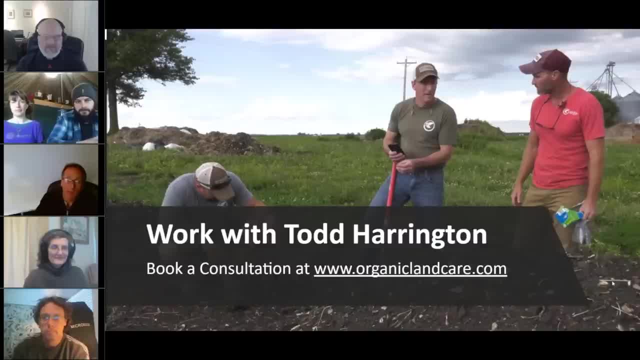 So you don't have to spend 250.. It's just in that situation, you know, it's difficult to try to use a sprayer. It comes to the, you know, applying that biology, the liquid part, it's very difficult. 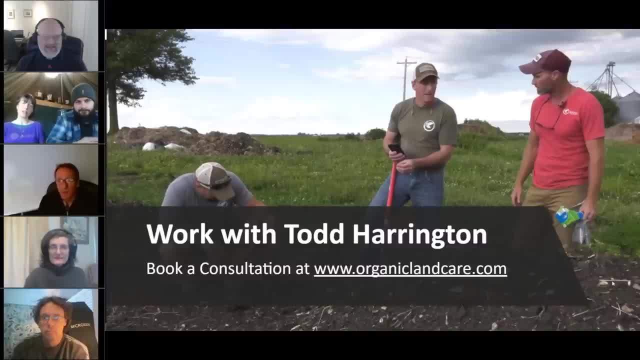 to use a conventional sprayer. But other than that there's a lot of modification. Yeah, Any creative ways that we have soiled food web, that we can adapt existing equipment. I'm sure Casey, you guys you know, have been able to do it. 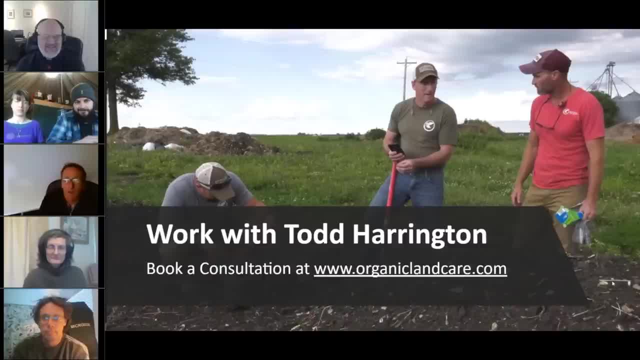 Brian and Wes. you know, there's just so many different ways that we can modify these smaller sprayers out there And that might not have been used with chemicals and so on and so forth. Yep, So people who are interested in large scale growers. 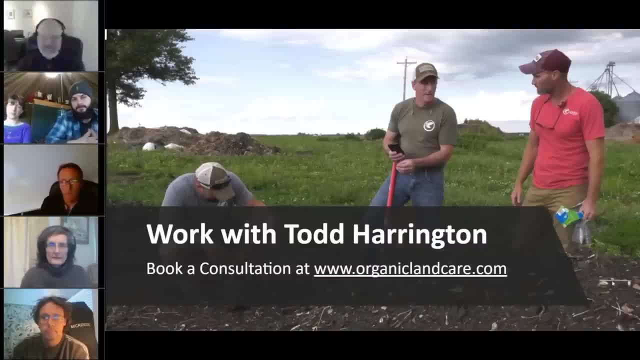 they've got a large scale, a lot of different questions that they can answer, And if you're looking for a large scale grower that they wanna work with, then they should be coming and talking to you, because you've already been through this process. 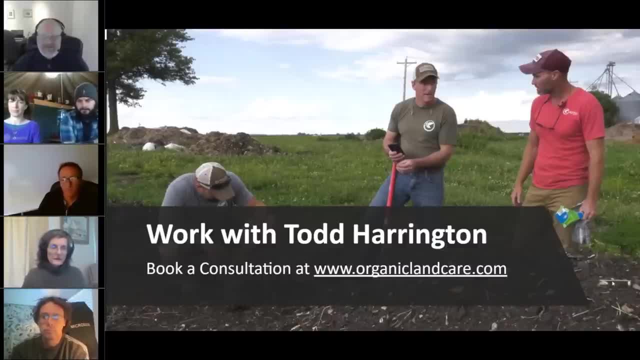 and you know some of the pitfalls, some of the things you have to say. So I think some of our folks going thinking about being consultants, they need to have you as a consultant for a year or two, while all of this conversion of the equipment has to happen. 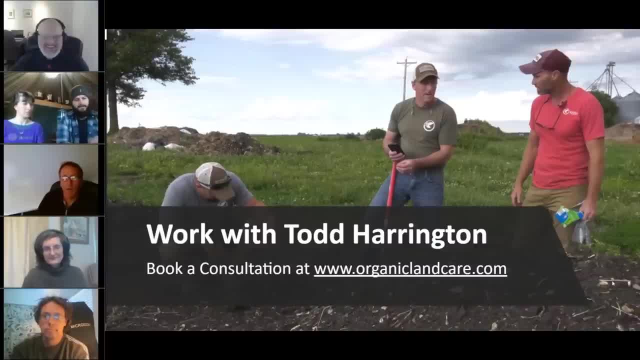 Exactly, Yeah, Yeah, Yeah. I mean there's something to be said about it, to be said about world-class experience, but plenty of us that have gone through it that can help people that are on this webinar. prevent you from making the same. 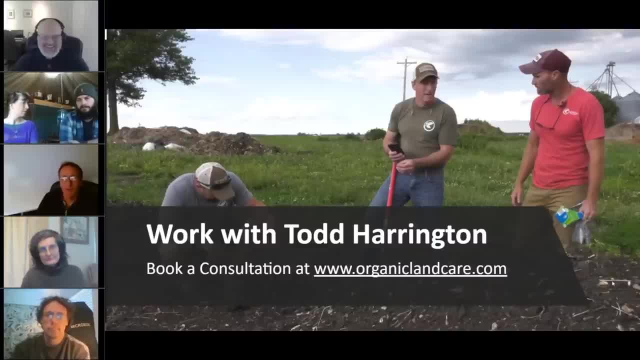 mistakes we might have made. if we've all made funny mistakes, that's how we learn and we will continue to make mistakes. but as a collective group that has gone through this, it's not like we started yesterday. you know the lane. I know I started working with you in the late 90s. I mean we've got decades of experience. 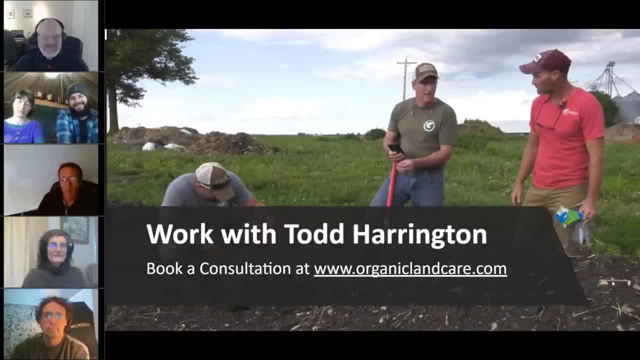 and mistakes, that we can help prevent that from happening, with a lot of people getting involved. that's one of the reasons for the course, really, yeah, it is really. you don't want to have to go out and reinvent everything from the ground up- haha, sorry, puns. you want to take somebody else's experience and not make. 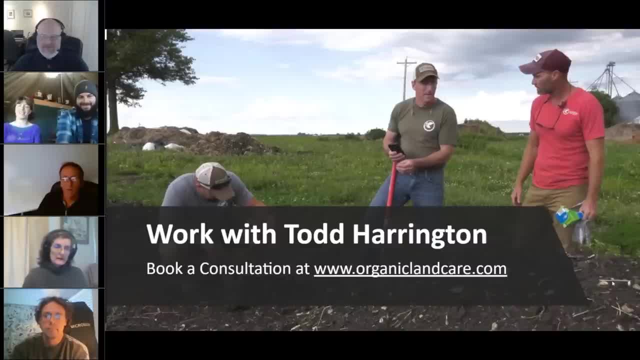 those mistakes and hopefully we'll be able to guide people and how do you actually really make this work? and it's a lot less expensive for the grower ultimately than the chemical approach. but I want to say to the entire group is extremely important, extremely important when we're working on this kind of a scale. we can't. 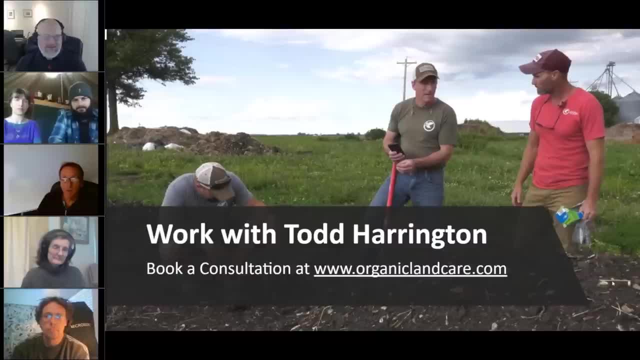 afford to make mistakes, and that is the reason for the foundation course. we need to know exactly what we're looking at and we need to know that we have systems in place that we're not going to produce ecoli and spray it out on the entire. 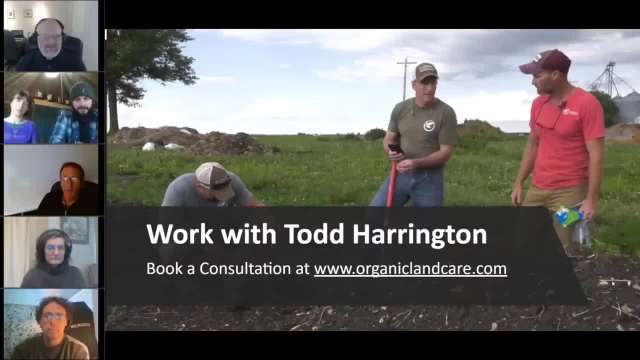 field that can't happen and it won't happen. and that's another reason for you know, really promoting the course here is that it will prevent us from making those kind of mistakes, instead of just going out and being those like the Wild West out there and saying I'm gonna take this aged manure and I'm gonna go. 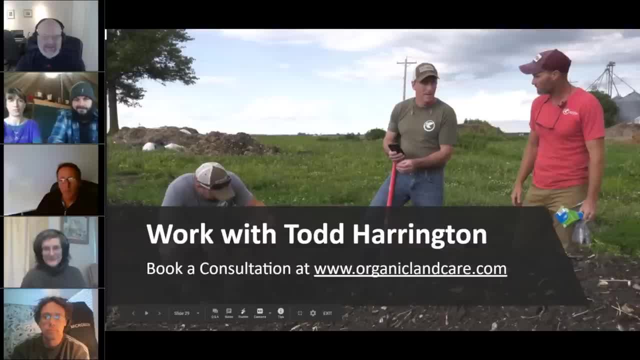 spray it out. so yeah, for sure, I think a big compost he's kept. these days, a lot of people just load them with foods and then spray them out on crops and this is like: no, you gotta go way off that stuff. you can make things go haywire like this.